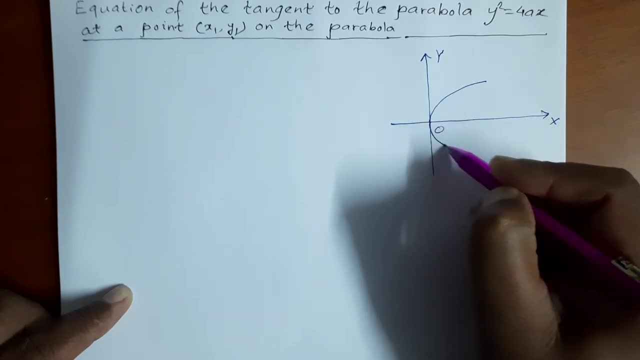 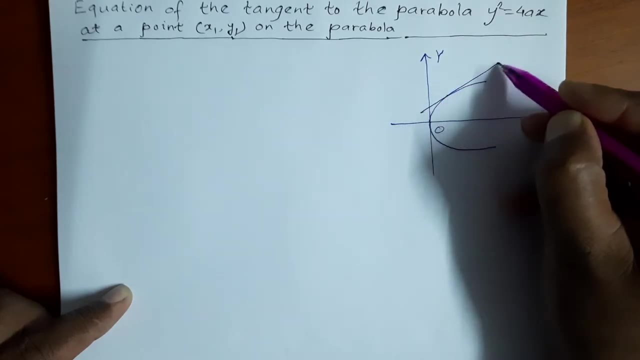 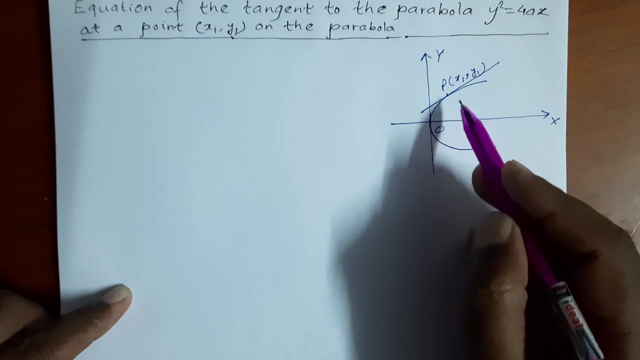 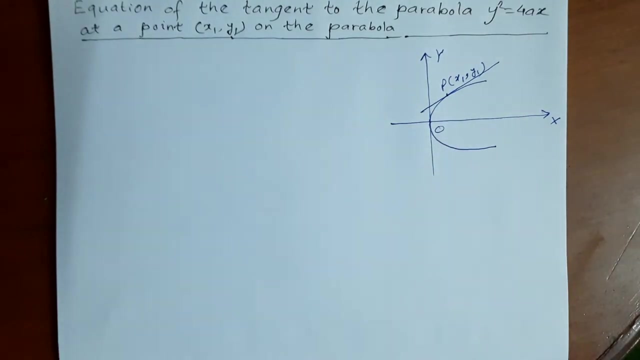 So its graph is like this, and suppose there is one point here: p, x1, y1.. So this is the tangent aligned to the parabola at this point: p. Now we need to find out the equation of this tangent line. Suppose it is ab. equation of tangent. 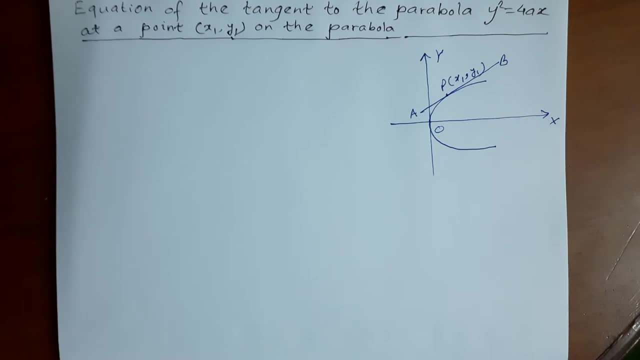 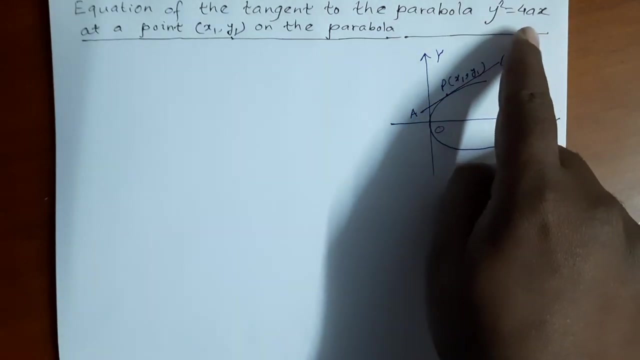 ab. So we have to find out, and we know that the slope of the tangent is given by first derivative dy over dx. So first of all we will differentiate y square equals to 4x and find out dy by dx. that gives us the slope of the tangent. okay, at any point on the curve. 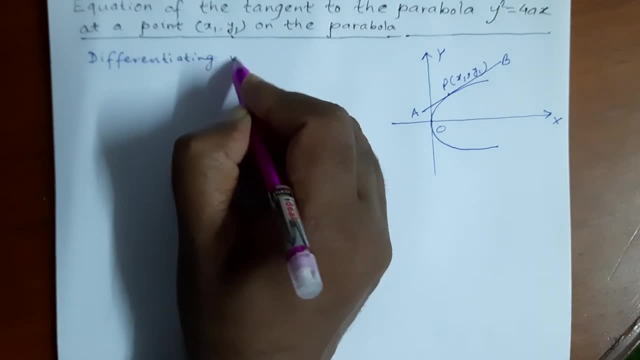 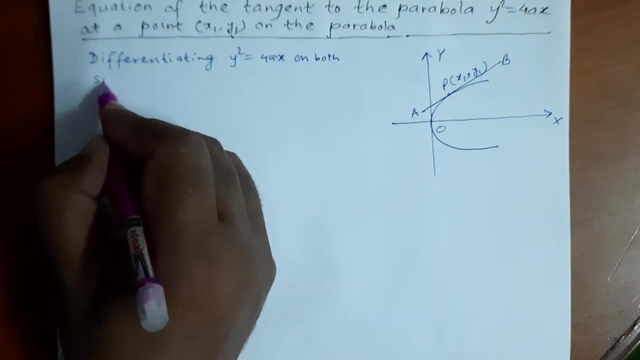 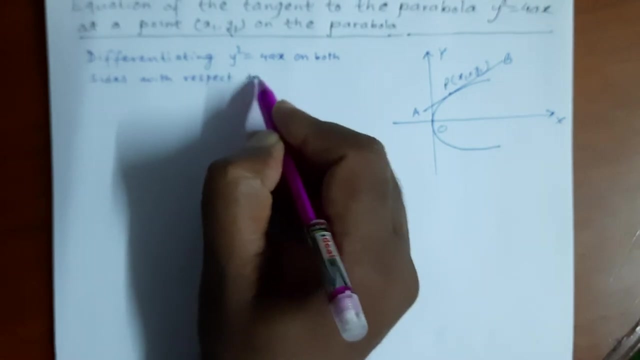 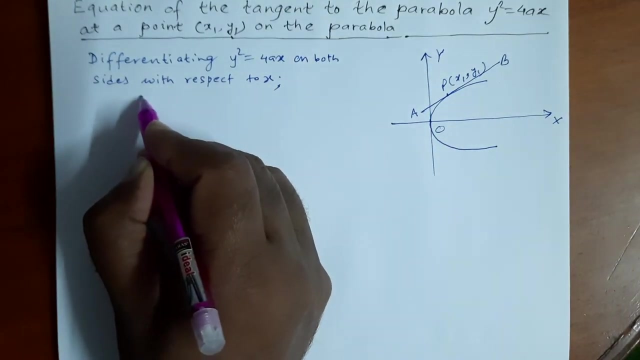 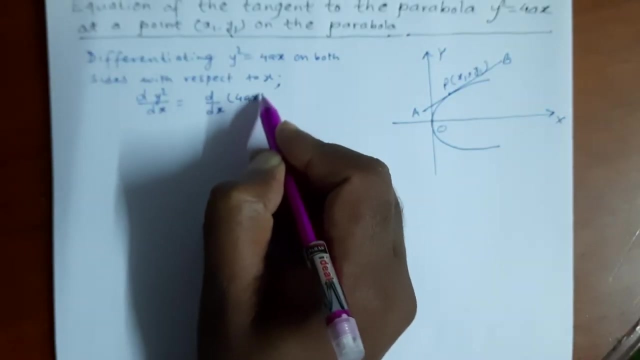 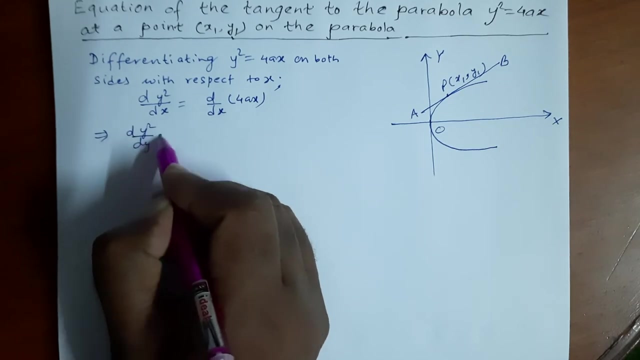 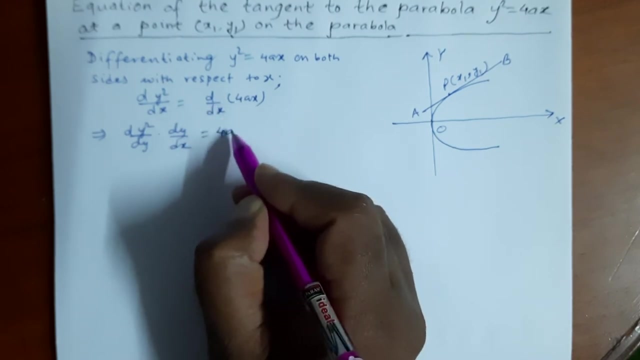 Differentiating the tangent by taking polar inverse y square and taking polar inverse over dx, you will find that dy, defined by dy, ordinary square on zy, phoe x. and now we can make the change, for this dy square over dy and dy over dx equals to phoe, dx over dx, this phoe x constant. we can write here dx over dx, that the value is one. 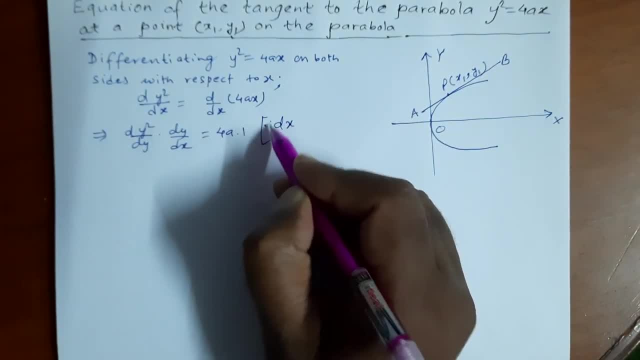 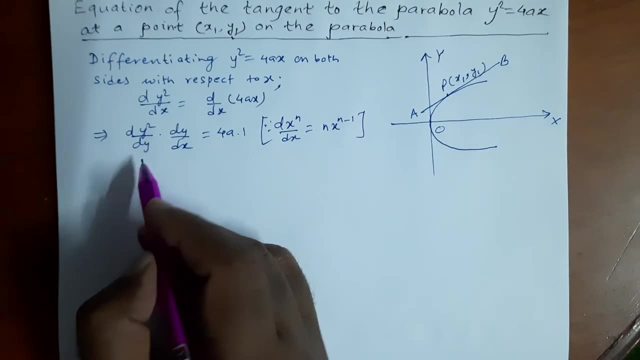 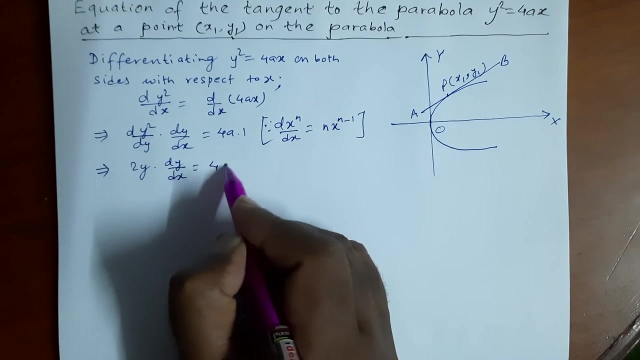 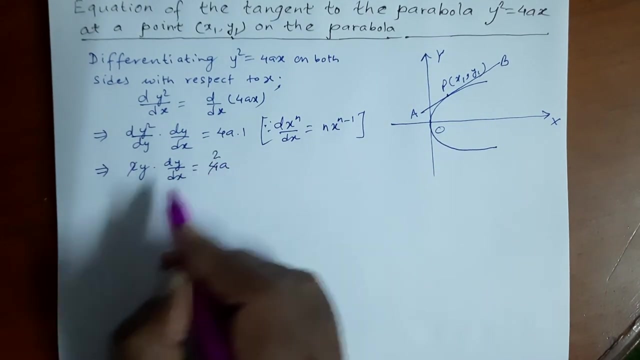 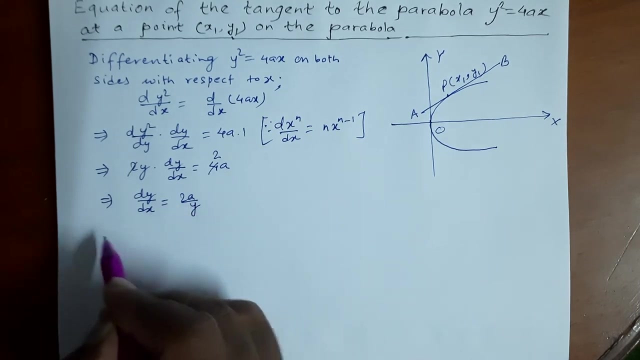 and you know that dxn over dx, its formula is nx and minus one. so using that formula, dy square over dy will be 2y, and here dy over dx equals to phoe and the phoe. and now this two can cancel this four. two two's are four. this implies dy over dx equals to 2a over y. therefore slope of tangent. 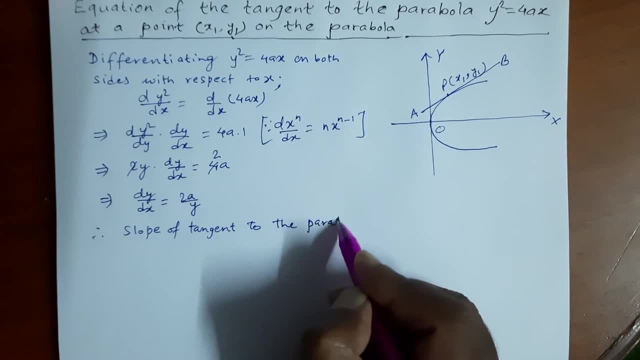 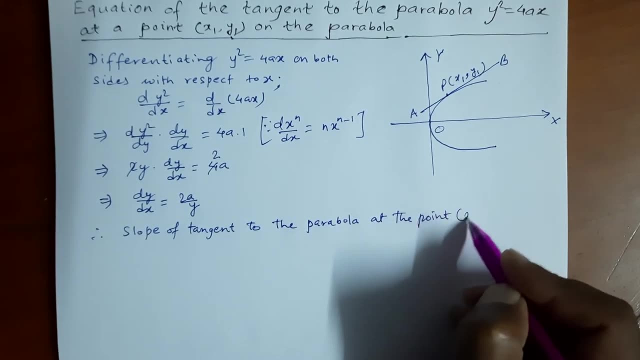 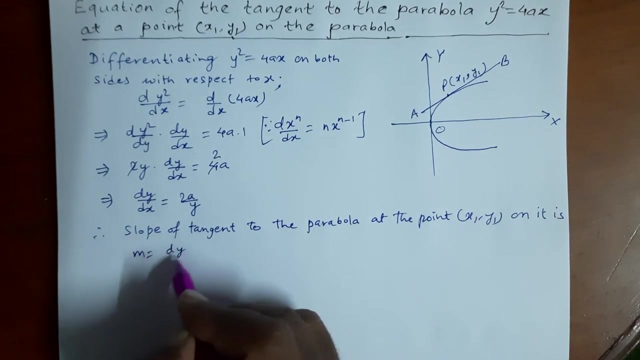 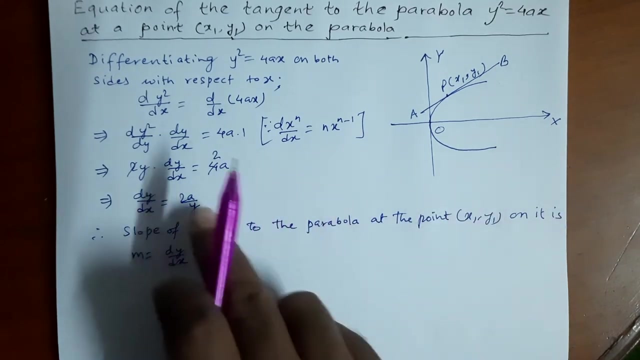 the parabola. parabola at the point. at the point x1, y1 on it is m equals to dy, by dx, equals to 2a over. in place of this, 2a over y, we can substitute x1, y1. there is no x, so this: in place of y we can put y1, so 2a over y1. 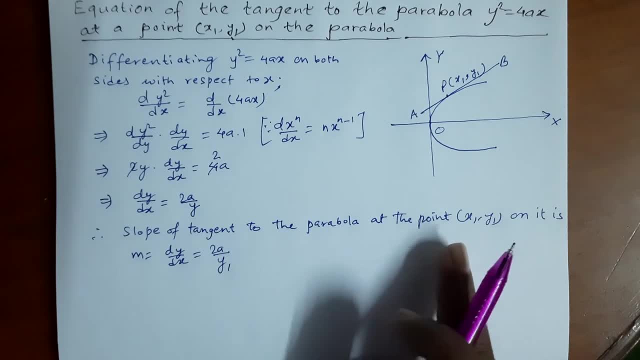 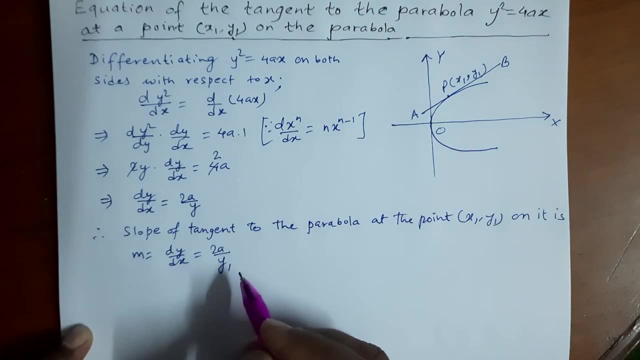 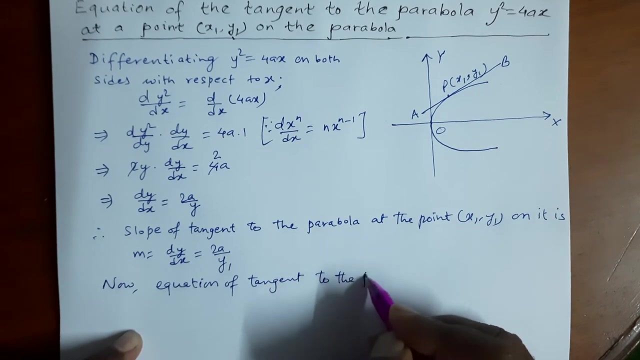 the slope of the tangent to the parabola. at the point x1, y1 on the parabola, and we know equation of the straight line in slope intercept form is: y minus y1 equals to m x minus x1. now equation of tangent is equal to the. 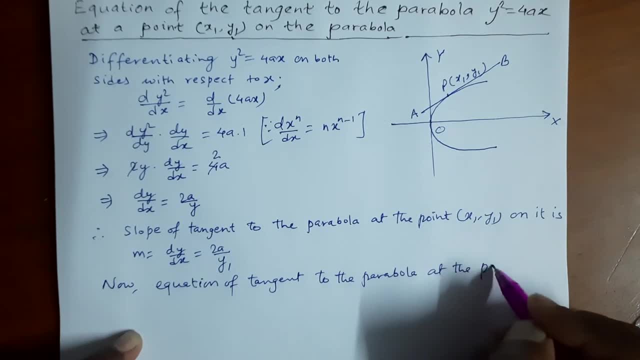 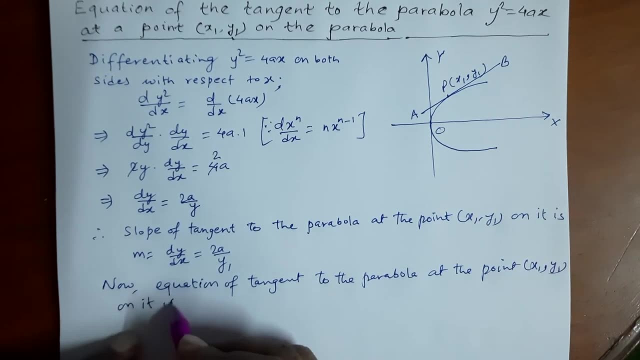 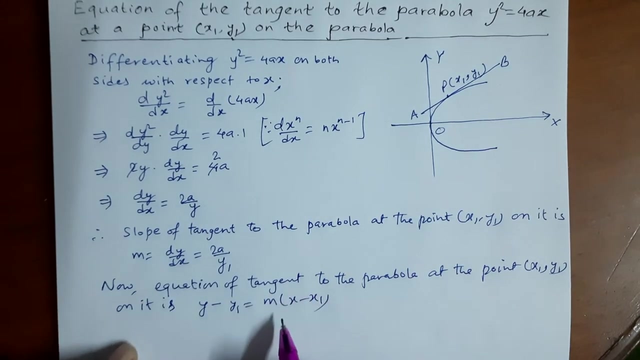 parabola at the point on it is: y minus y1 equals to m, x minus x1.. This is the equation of straight line in point slope form. So this m can be replaced by 2a over y1 because slope of the tangent is 2a over y1, we will do that y minus y1 equals to m is. 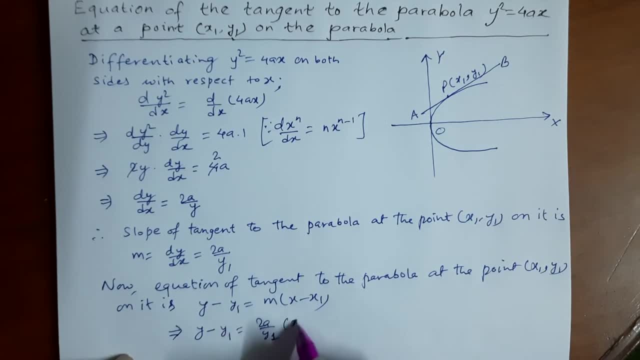 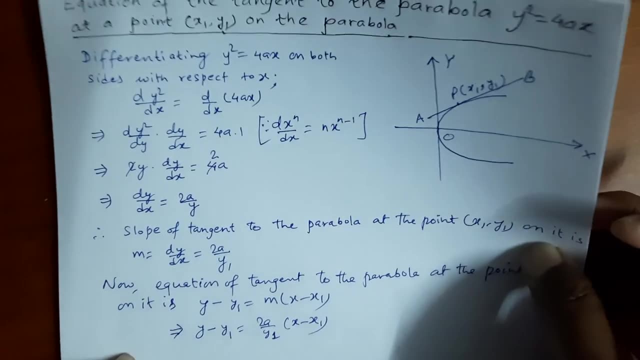 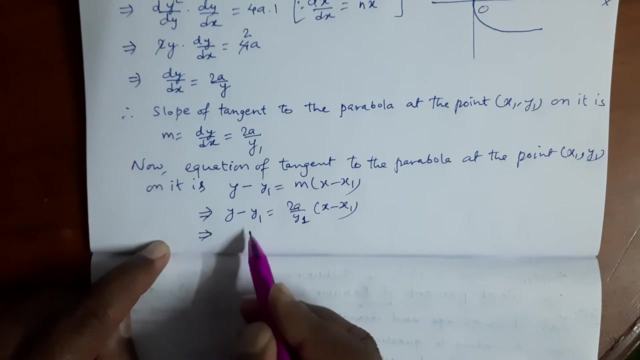 2a over y1, x minus x1 is here, and now we can cross multiply. this implies y times y1, y1 minus y2.. y1 times y1,, that is, y1 square, equals to 2a x minus 2a x1.. And as you know that the point x1, y1 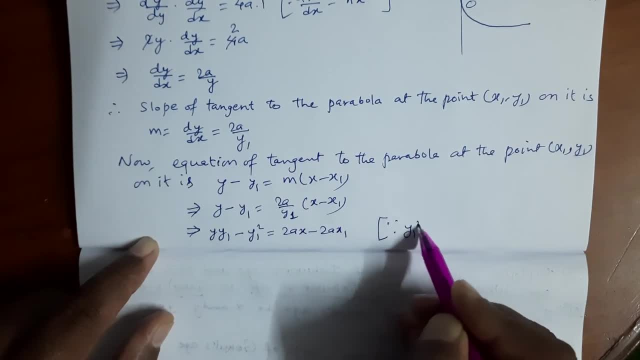 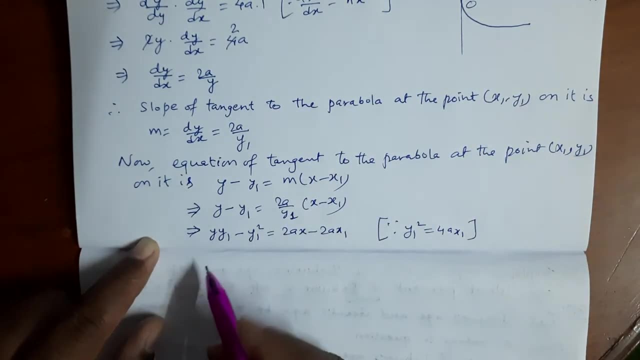 lies on the parabola, so y1 square equals to 4a x1, because x1, y1 lies on the parabola, So in case of y1 square we can write 4a x1.. This implies y1 minus 4a x1, equals to 2a x minus 2a x1.. 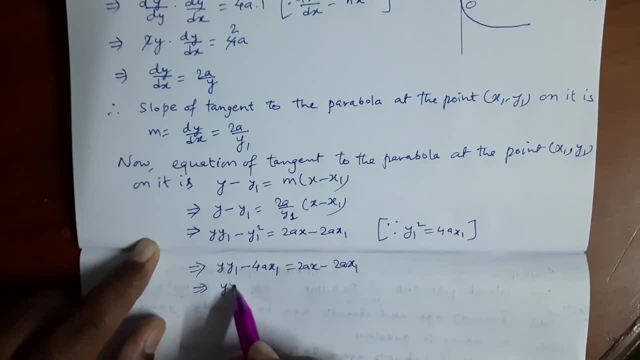 And this implies y1 equals to 2a x minus 2a x1.. This minus 4a x1 goes to other side and becomes plus 4a x1. This implies y1.. y1 equals to 2a x. this 4a x1 minus 2a x1 is plus 2a x1. Therefore, yy1 equals to 2a. 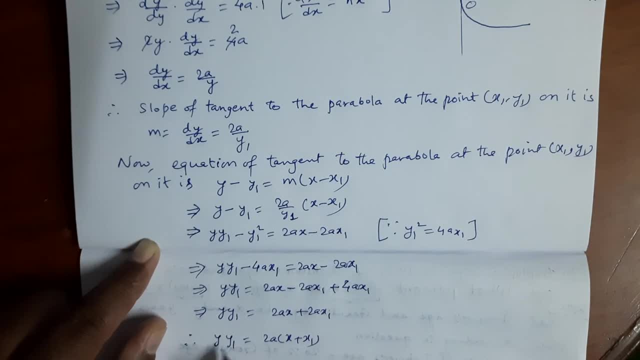 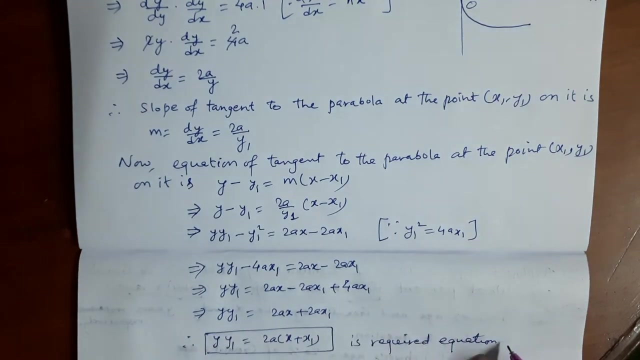 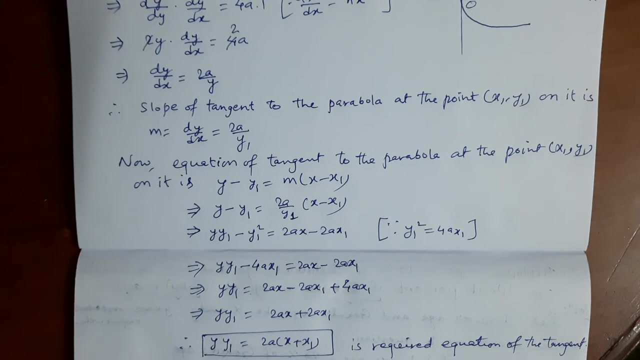 x1 is common, x plus x1 is required. equation of the equation of the of the tangent to the parabola at the point x1, y1 on the parabola. okay, So So we have two equations of the parabola, one equation of the two. equation of the tangent. 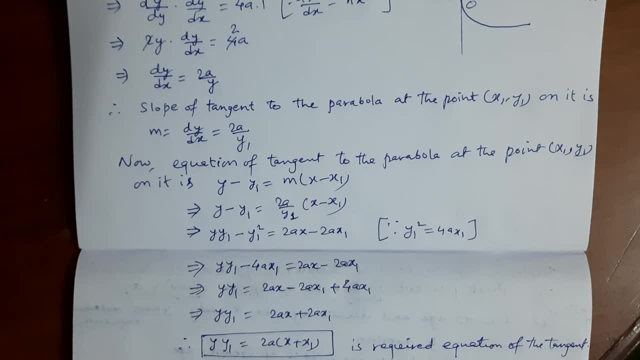 to the parabola. one equation of tangent to the parabola was: y equals to mx plus a over m, and this is: yy1 equals to 2a x plus x1, okay, So if the point is given, then we need to use this equation of the tangent to the parabola. 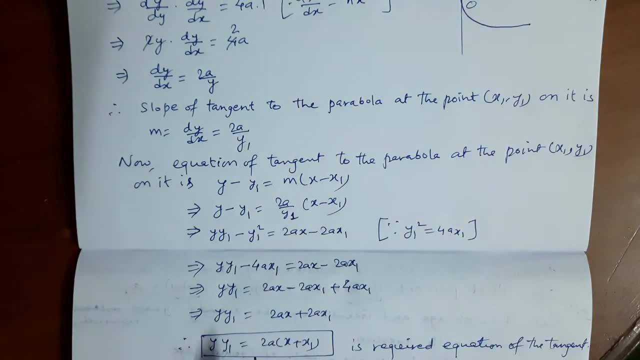 yy1 equals to 2a x plus x1.. If point on the parabola is given, then we should use this equation: yy1 equals to 2a x plus x1.. Okay, And if the point on the parabola is not given, point outside the parabola is given, or point. 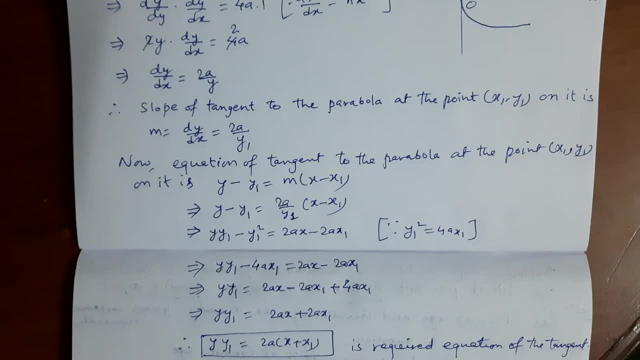 not given at that time, we should use y equals to mx plus a over m as the equation of tangent. So I hope that you understood in which case we have to use equation of this tangent to the parabola and in which case we have to use y equals to mx plus a over m as the equation. 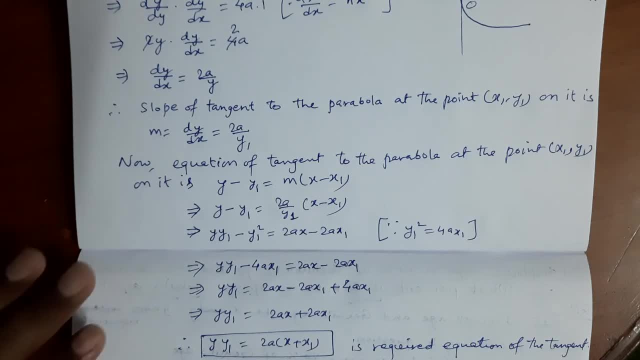 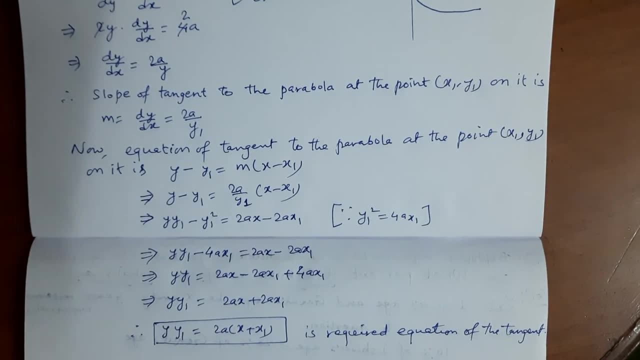 of tangent to the parabola. And now, similarly, using the slope of this tangent to the parabola, we can also find out equation of normal to the parabola. okay, equation of normal to the parabola at a point. 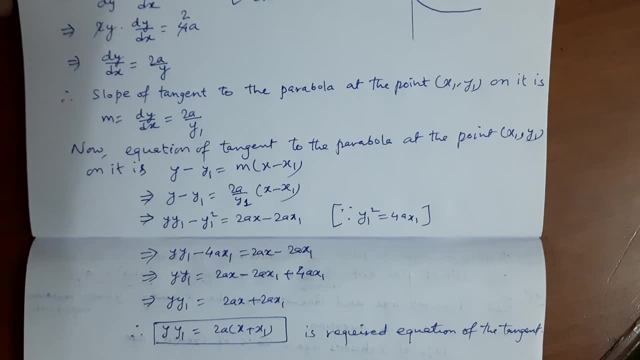 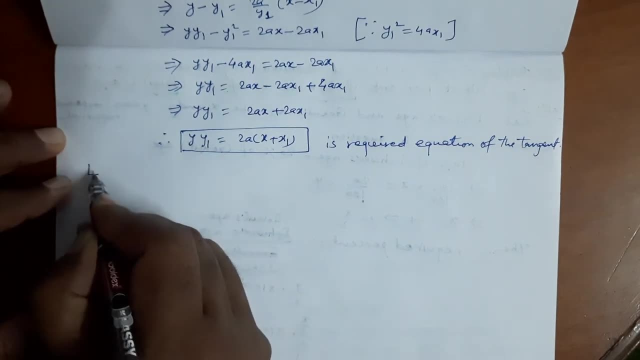 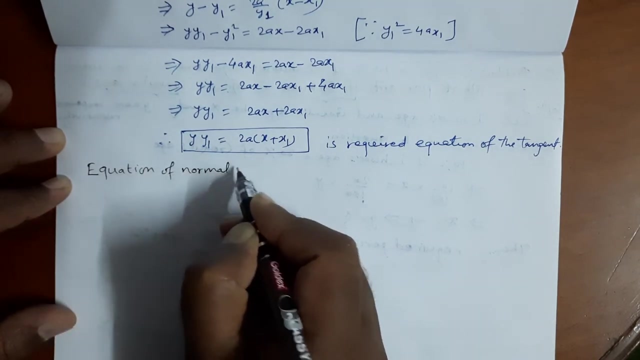 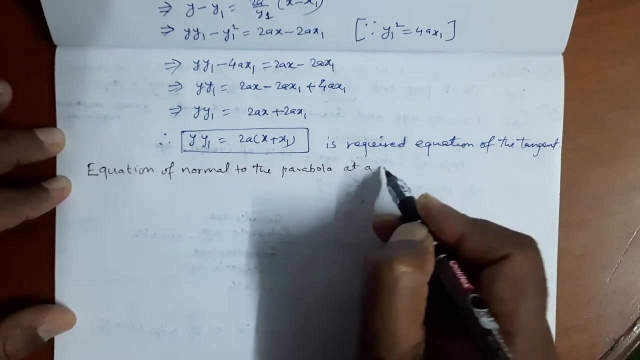 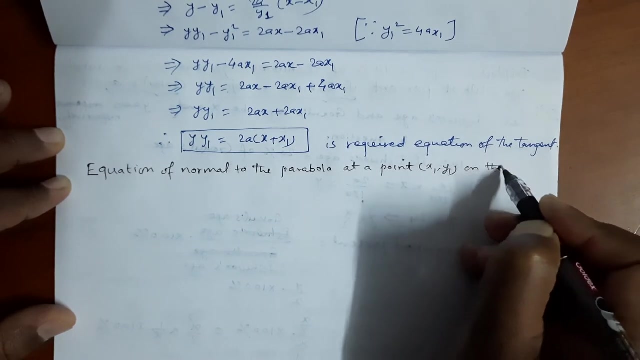 x1, y1 on the parabola. okay that. So we have to use equation of normal to the parabola. okay. equation of normal to the parabola at a point x1, y1 on the parabola. okay. equation of normal to the parabola at. 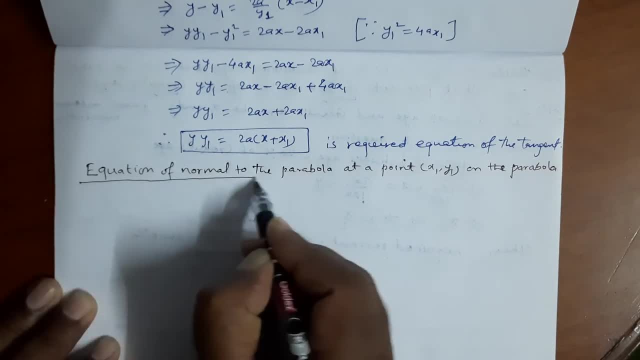 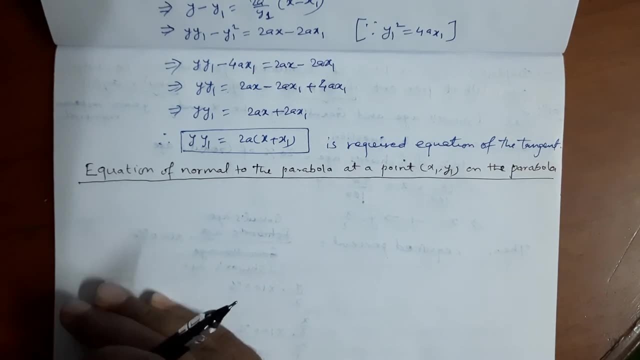 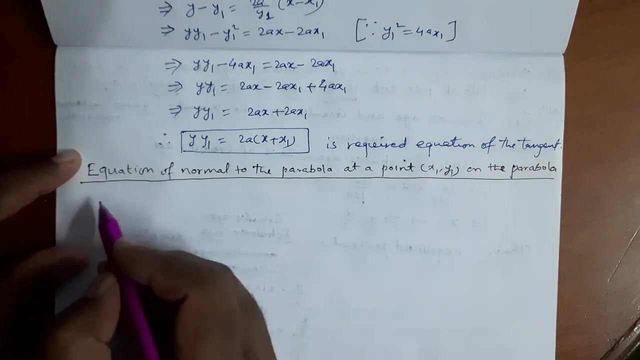 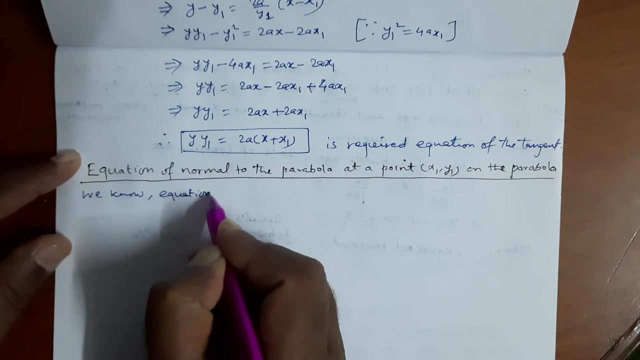 a point x1, y1 on the parabola. okay, Now we know equation of the tangent to the parabola is the derivation of this. we know equation of tangent to the parabola is: we know equation of tangent to the parabola at: 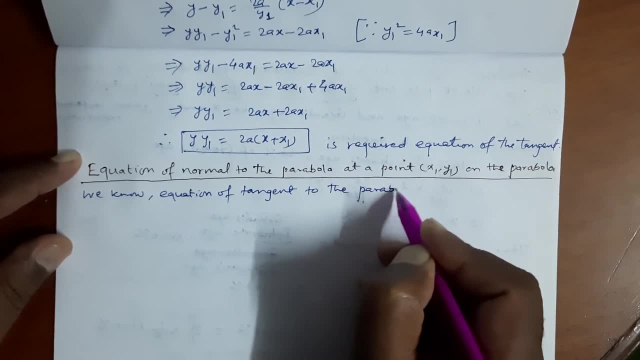 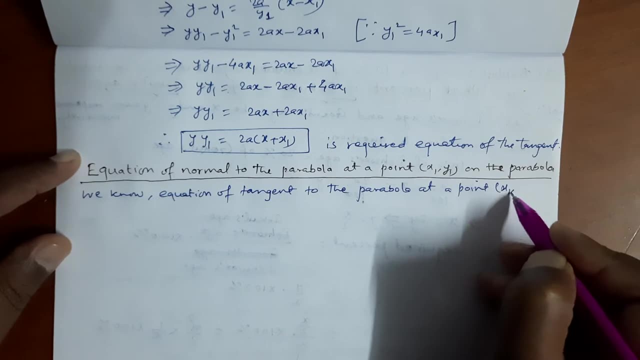 the point x1, y1 on the parabola. Now we know equation of the tangent to the parabola at a point x1, y1 on the parabola at a point x1, y1 on it is yy1 equals to 2ax plus x1. and now slope of the tangent. 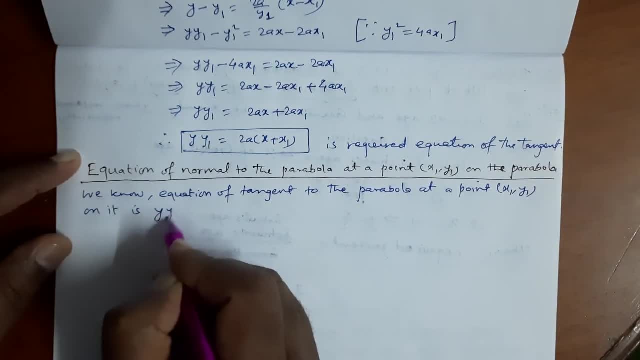 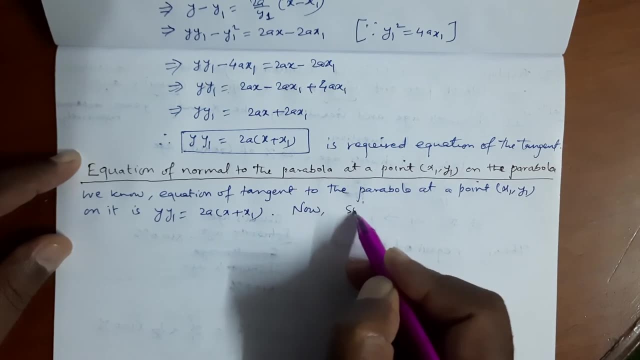 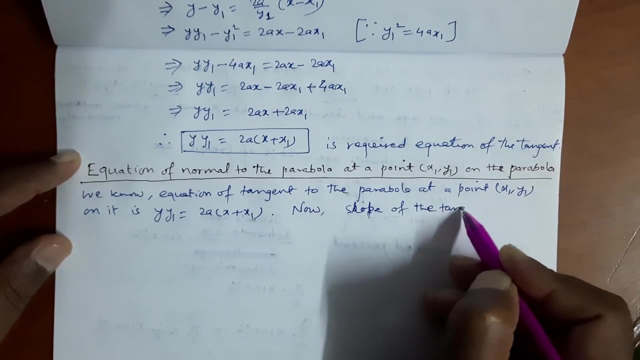 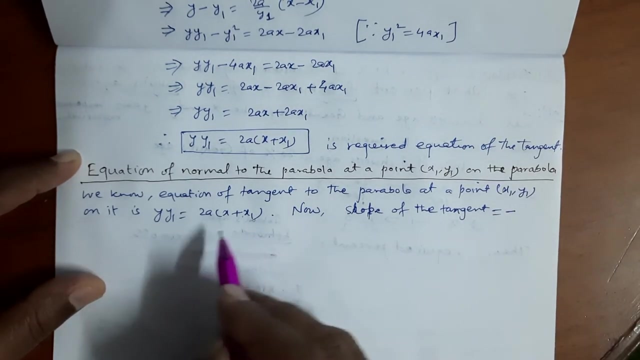 to the parabola. at a point x1, y1 on it is yy1 equals to 2ax plus x1. and now slope of the tangent. slope of this tangent equals to minus. here slope of the tangent is 2a. 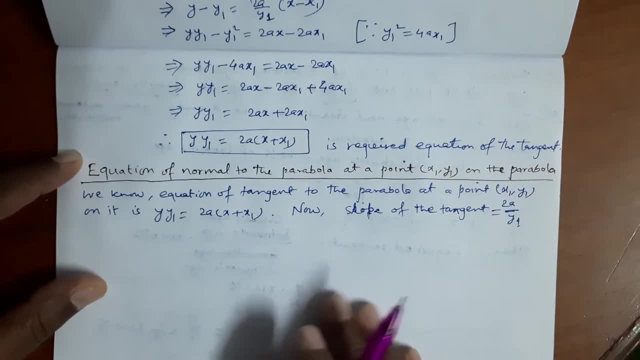 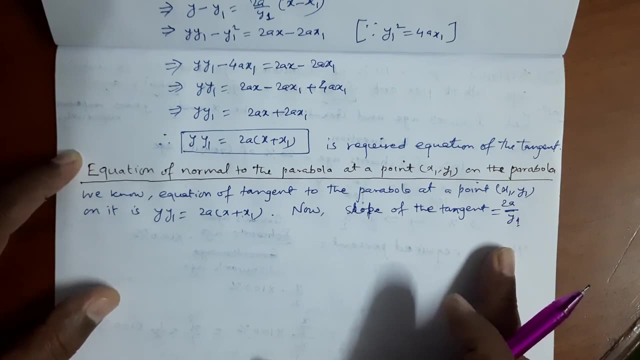 over y1,. okay, slope of the tangent is 2a over y1 and since the tangent and normal are perpendicular to each other at the point of contact, so slope of the normal equals to, therefore, 2a over y1.. 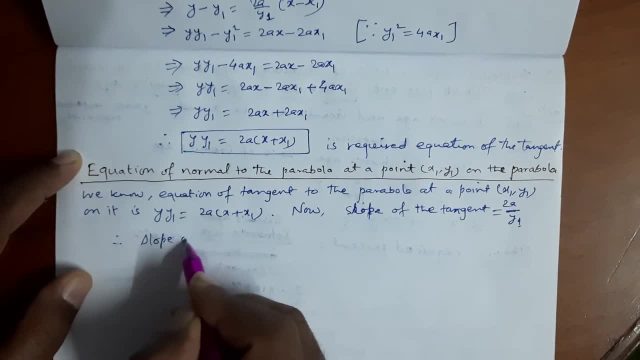 So slope of the tangent is 2a over y1.. So slope of the tangent is 2a over y1.. So slope of the tangent is horizontal and horizontal shorter than 2a over y1.. So slope of the tangent is 2a over x1 and horizontal shorter than 2a. 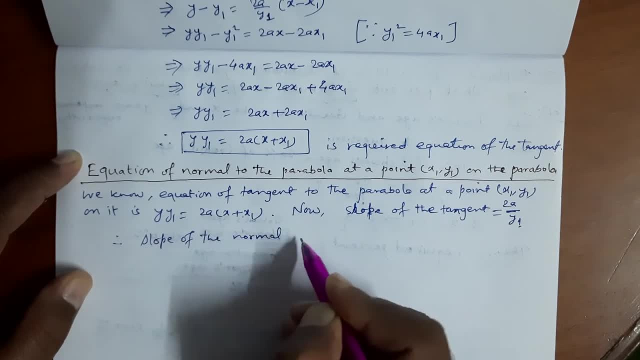 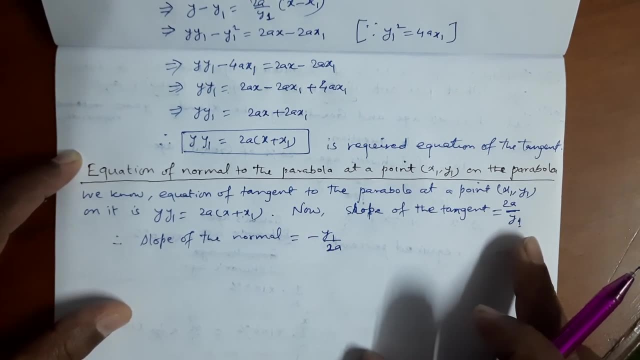 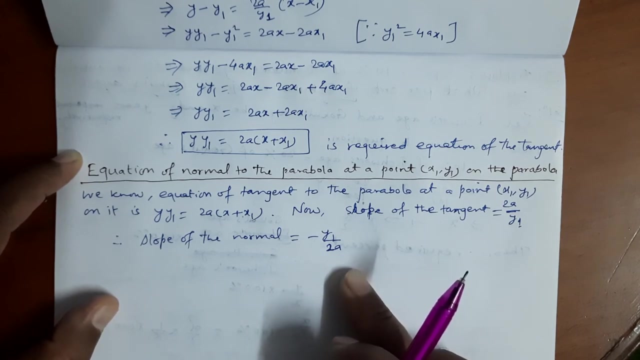 We have taken here this so that slope of the tangent and normal becomes minus 1, here if you multiply this you will get minus 1, so we have taken its reciprocal and equal to equal sign so that product becomes minus 1, because slope of the tangent and product. 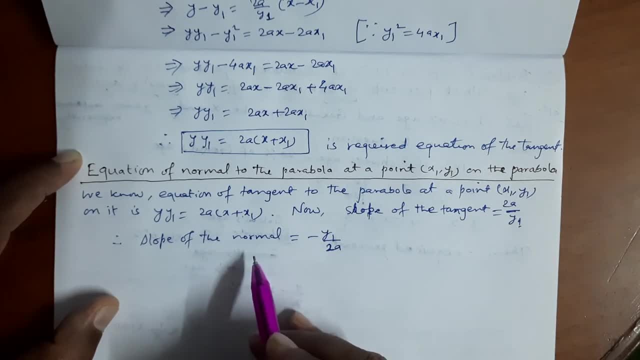 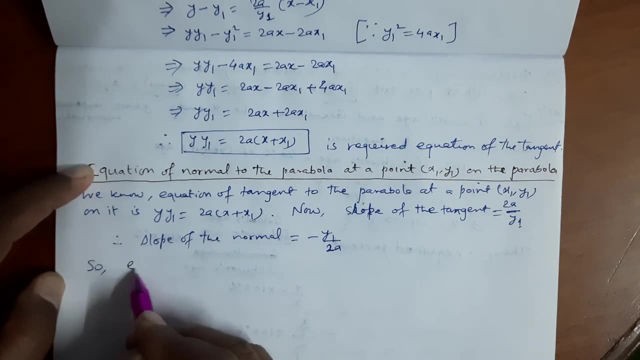 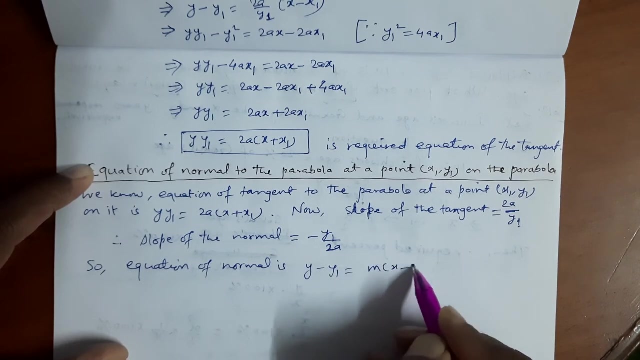 of the slope of the tangent. and nou, and tangent is opposite, normal is minus 1.. And so equation of the normal is equation of normal is. we use point slope form, that is, y minus y1 equals to m, x minus x1, here m is the slope of. 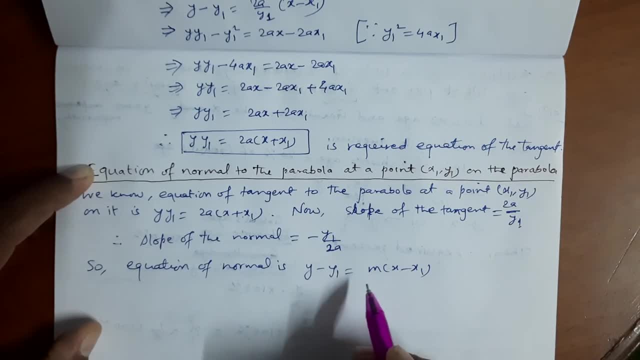 the normal. so we substitute slope of the normal in place of m, so m equals to. we put minus y1 over 2a y. minus y1 equals to minus y1 over 2a x minus x1.. This is the slope. 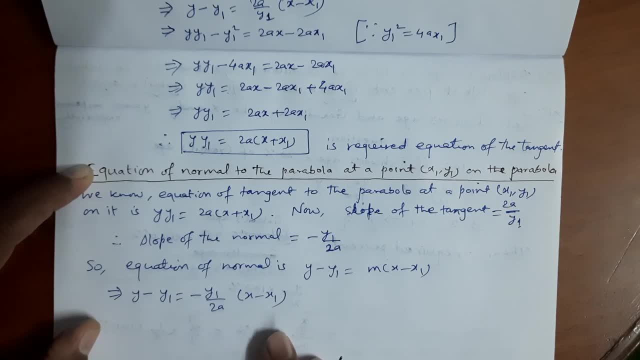 this is the equation of the normal. okay, if the point x1, y1 and the equation of the parabola is given, y square equals to 4x is the equation of the parabola that is given And using this equation we can also find out equation of the normal in slope form To get: 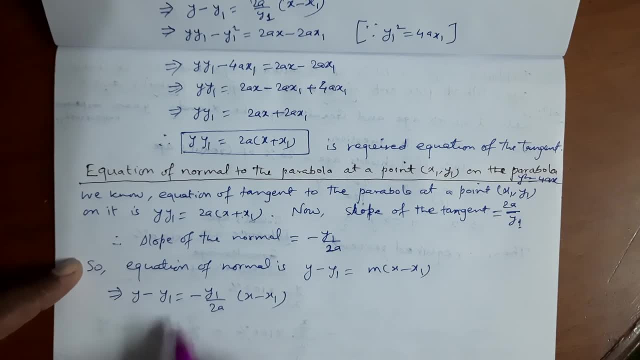 equation of the normal in slope form, we substitute: minus y1 over 2a equals to m. To obtain the equation of normal in slope form, we put: minus y1 over 2a equals to m. You substitute this And this implies y1 equals to and minus x1 divided by y1 equals to m. So if the point 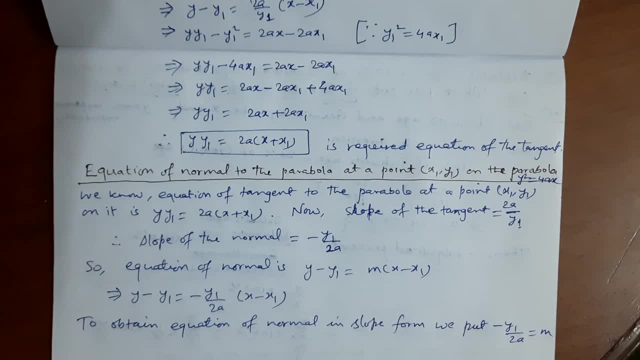 slope sobre y1. y1 equal to x2, and also this already, And there comes the angle that we meet ourpsyrtionしゃеля y1, beached here. So if that looks like so, then y2, x2, y2, x2,. 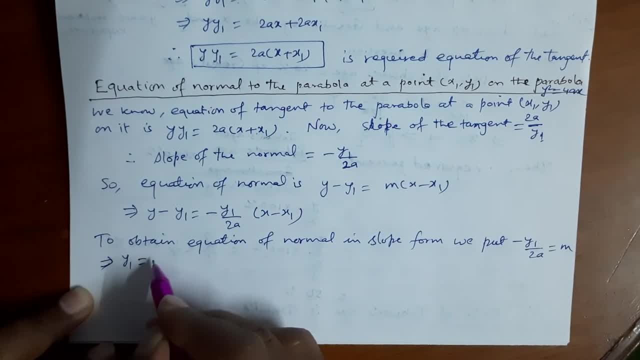 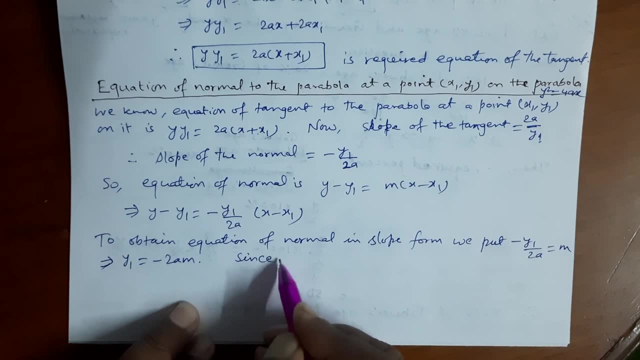 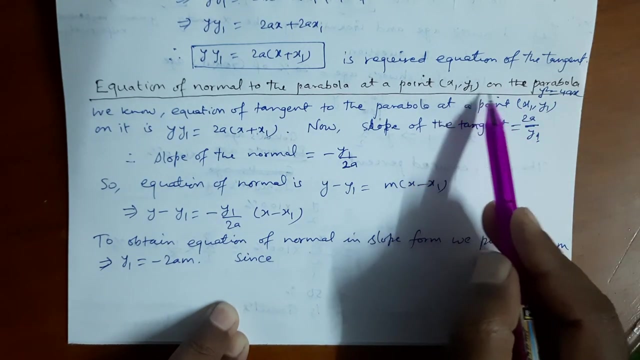 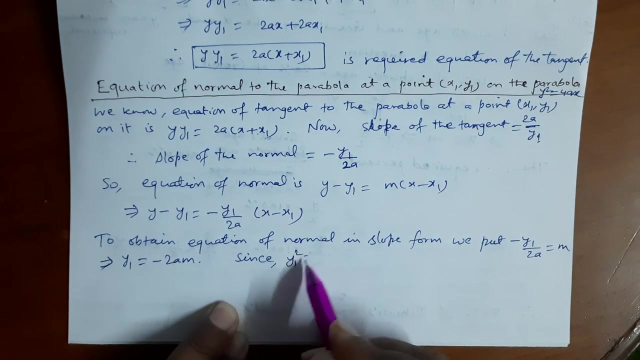 here also מs is one Jacksonさん, on the which we are also going to continue the same to minus 2 a m. okay, And since x1 y1 point lies on the parabola, y square equals to 4 x. this x1 y1 satisfies this equation of the parabola, So we can write: y1 square equals. 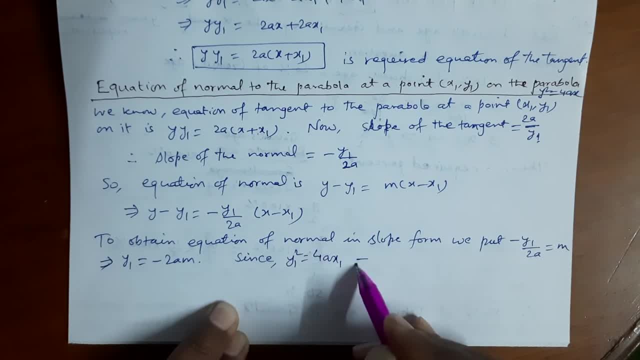 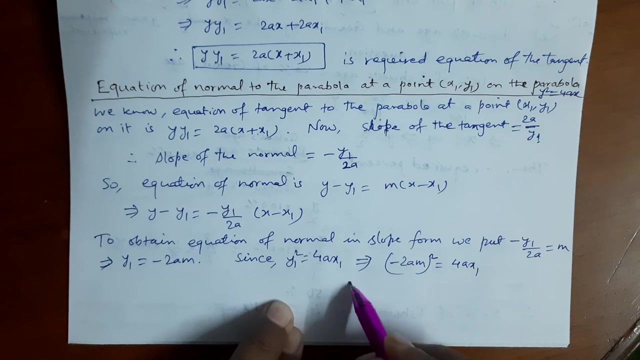 to 4 a x1.. This value of y1 we can substitute here, so we get minus 2 a m and its square equals to 4 a x1.. Now this implies minus 2 m Square that will be 4 a square. m square equals to 4 a x1. now 4, 4 can be cancelled and square cancels. So this implies 4 a square cancels too. So minus 4 a x1, cal've x0 equals to 4 m, or 4 m, which gave 4 a 1 minus 2 a square equals to 4 a x1. 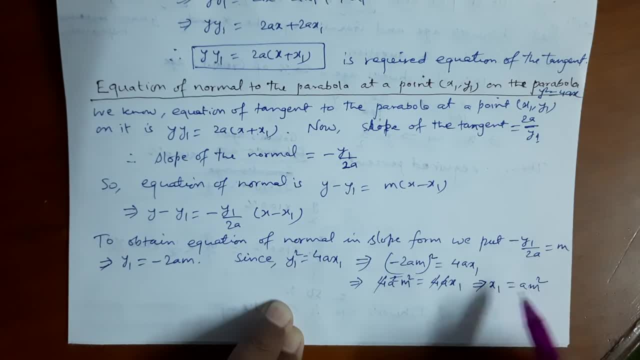 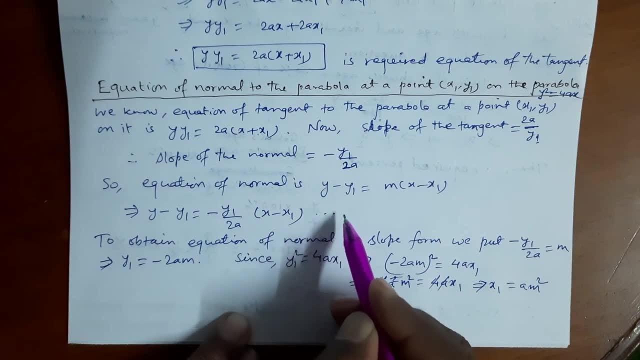 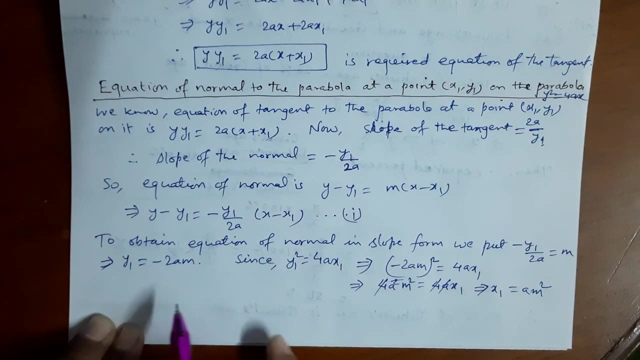 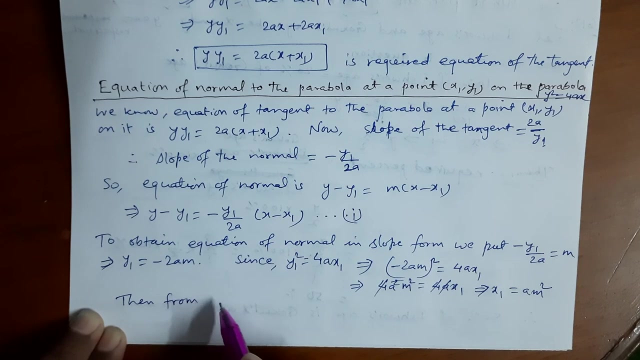 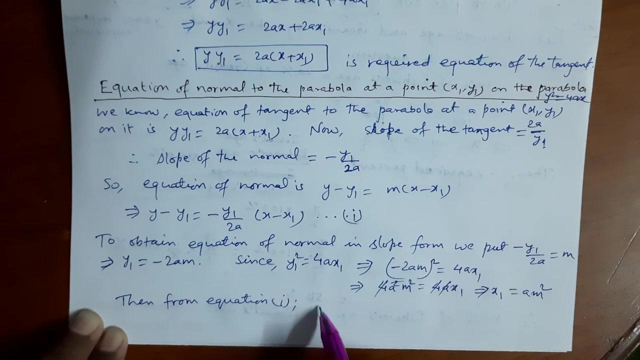 x1 equals to m square and you can call this as equation 1 and substituting value of x1 and y1 in equation 1.. Then from equation 1, y minus y1, y1 value is minus 2am. so this minus and this minus becomes plus plus 2am equals to: 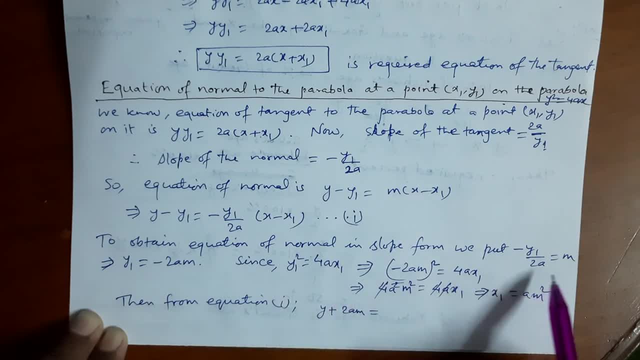 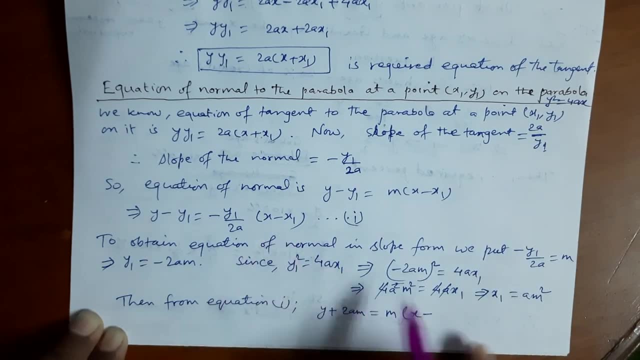 m square and you can call this as equation 1 and substituting value of x1 and y1 in equation 1.. Minus y1 over 2a, we have substituted m, so in place of m we can put m x minus in place of x1, from here we have got m square. so in place of x1 we can write m square. 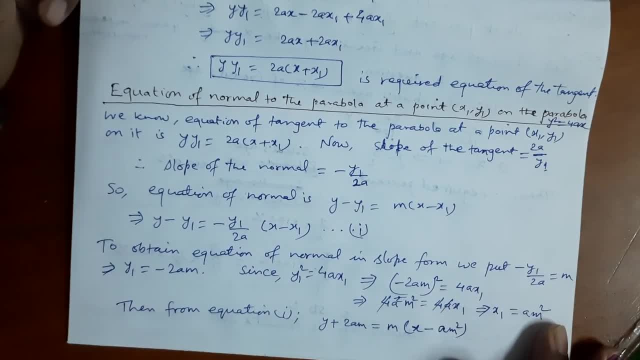 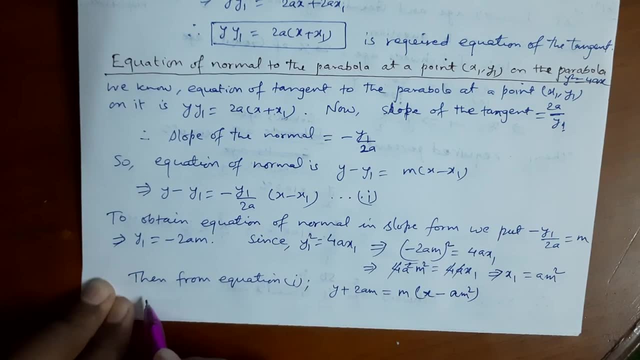 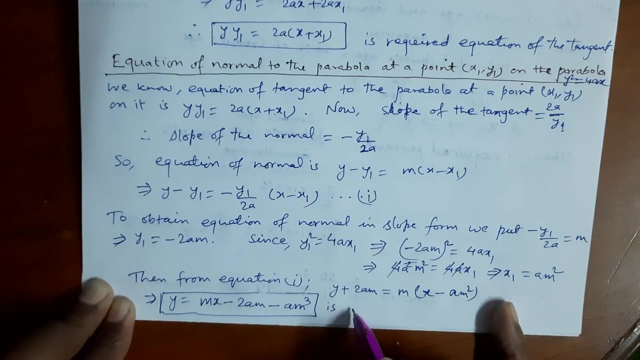 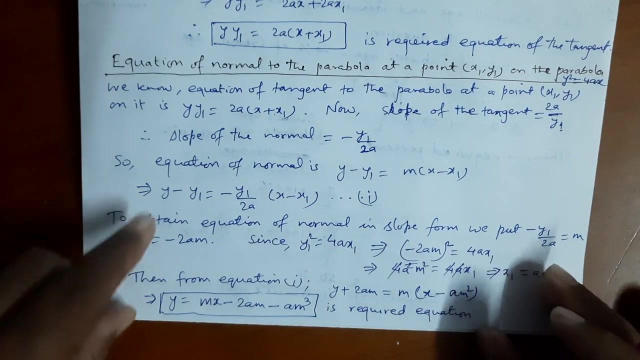 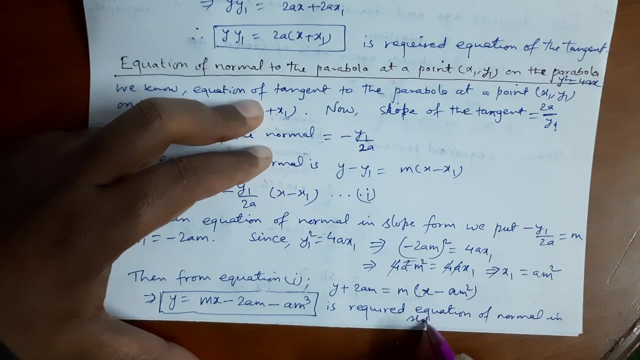 m square and now this implies y equals to mx. this 2m goes to other side, because minus 2m and minus mq, y equals to mx. minus 2m. minus mq is required equation of normal, of normal, of normal normal in slope form. So this is the required. 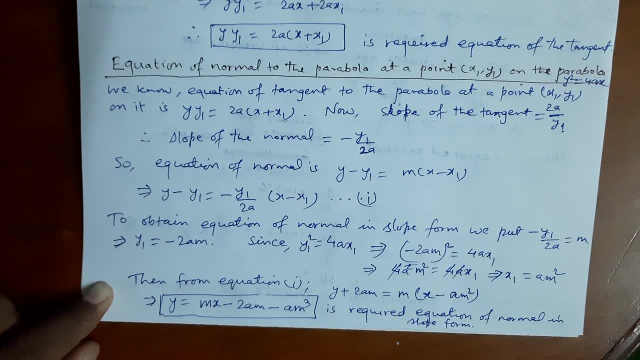 equation of the normal in slope form. So if slope m of the normal is given or we can find out, and if the equation of the parabola is given, then we use this equation of the normal to the parabola at the point x1, y1.. 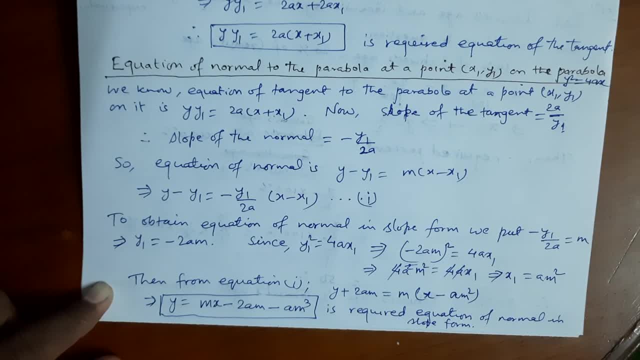 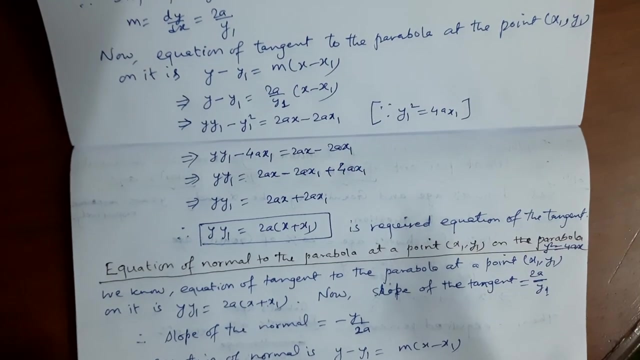 Okay, this way we can easily find out equation of normal. So in today's videos, I have taught how to find out equation of tangent and equation of normal. Okay, and if you need to copy this, you can pause the video and copy it. and Before I stop this video, I will tell you the technique to remember the formula of this equation of a tangent. 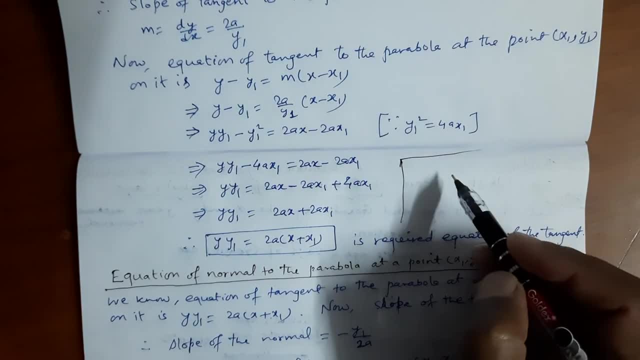 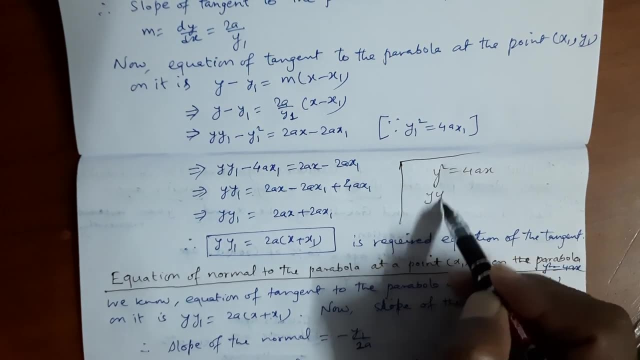 So here, to remember the equation of the tangent, we can do so. That is, y square equal to 4x is the equation of the parabola. So y square, we can add y times y. This 4x, we can add 2a times 2x. 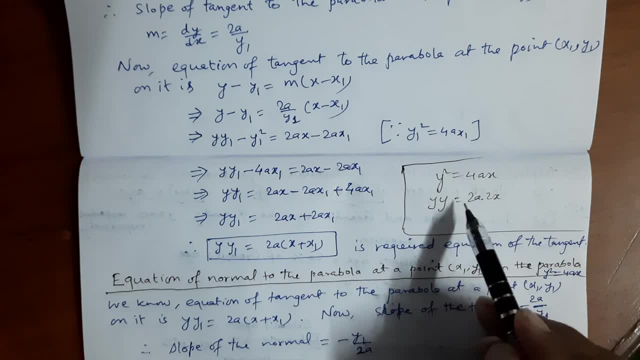 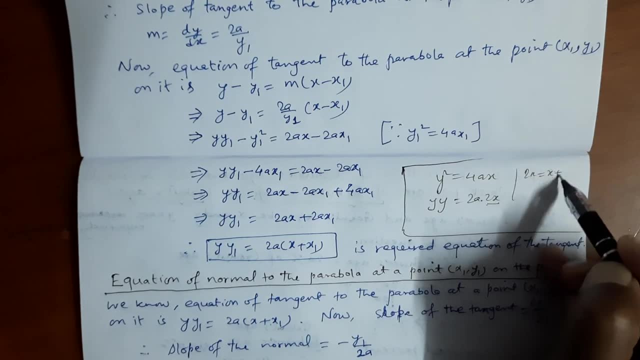 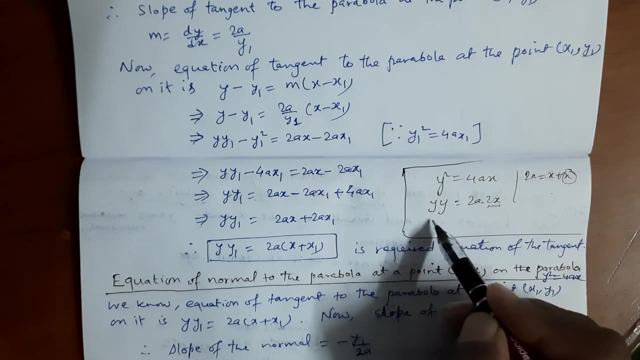 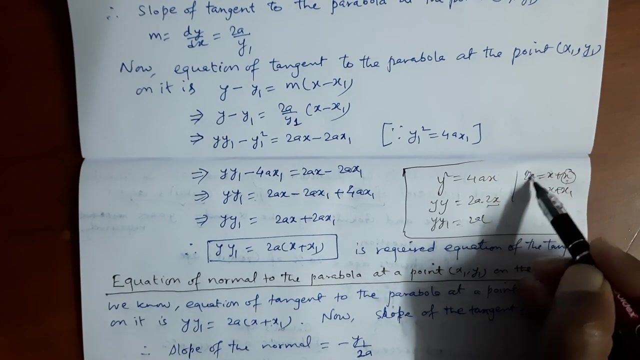 And if you just replace here y by y1 and this 2xy, 2x can also be written as x plus x And out of this 1x, this x can be replaced by x1.. So because yy1 equals to 2a, in place of 2x we can write x plus x1, replacing one of this x by x1..